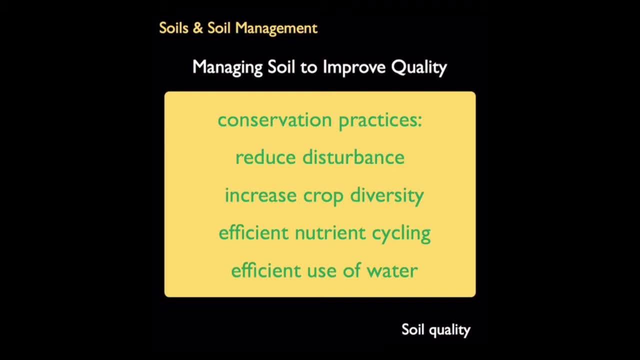 Managing soil. to improve soil quality entails the use of conservation practices that improve soil function In general. practices that reduce disturbance, increase crop diversity and efficiently cycle nutrients, water and energy will accomplish this. In my book, I discuss how to manage soil quality and soil quality. 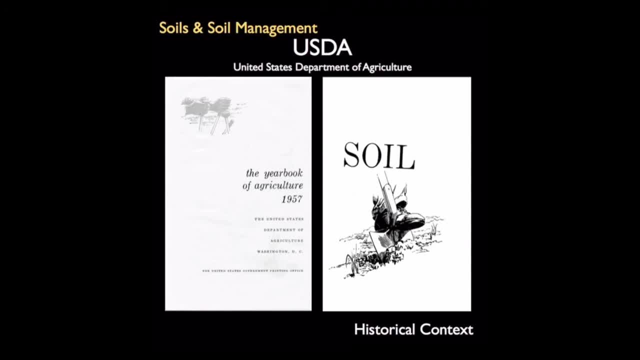 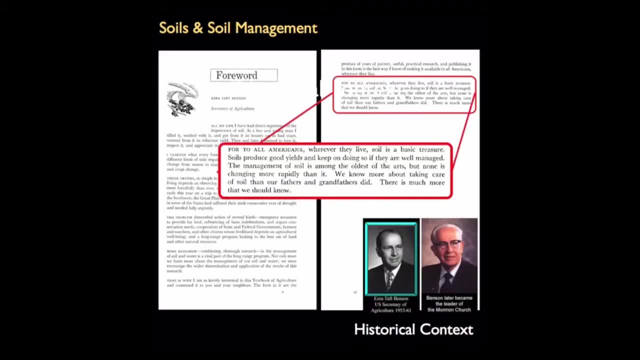 The 1957 USDA Yearbook of Agriculture was dedicated to the subject of soil. In the foreword to soil, Ezra Taft Benson, then Secretary of Agriculture, wrote: For all Americans, wherever they live, soil is a basic treasure. Soils produce good yields and keep on doing so if they are well managed. 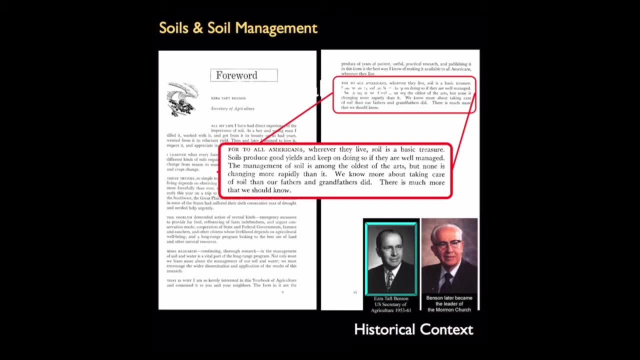 The management of soil is among the oldest of the arts, but none is changing more rapidly than it. We know more about taking care of soil than our fathers and grandfathers did. There is much more that we should know". His statement is as true. 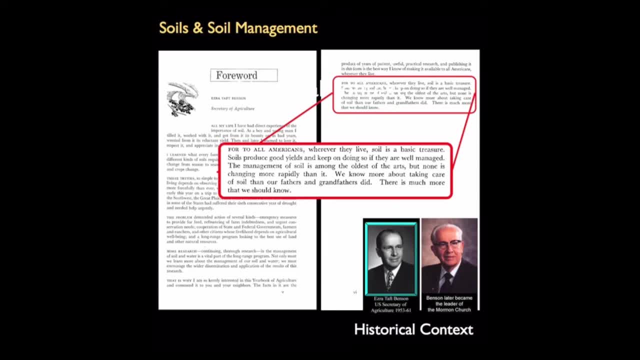 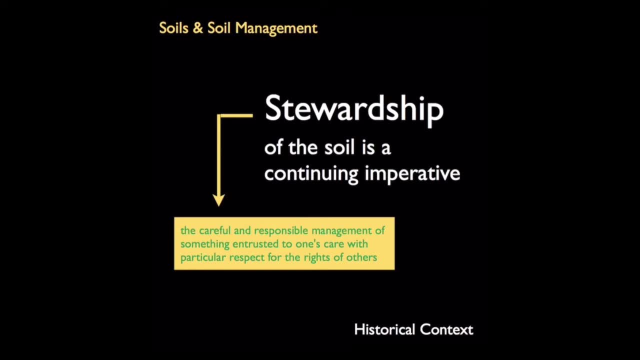 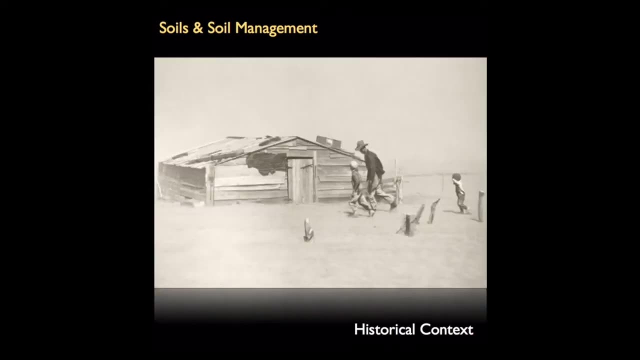 today, in the 21st century, as it was 50 years ago, Stewardship of this most valuable resource is a continuing imperative. The importance of high quality soils cannot be overstated. It was recognized in a dramatic way in the 1930s during the famous Dust Bowl events, Largely as a response to the devastating 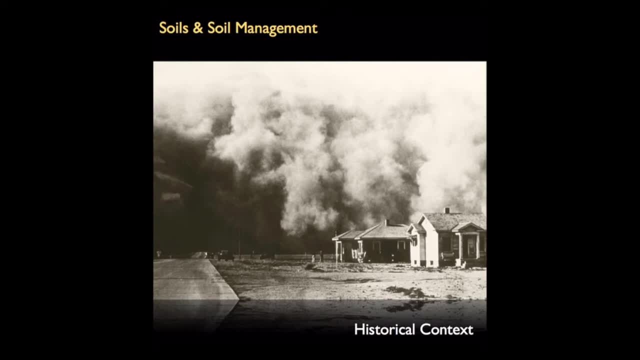 Dust Bowl years. in 1934, the United States Congress created a permanent federal agency, the Soil Conservation Service, to safeguard the nation's soils resource. This agency was initially charged to collect and analyze data about soil erosion, its causes and its severity. It was also responsible. 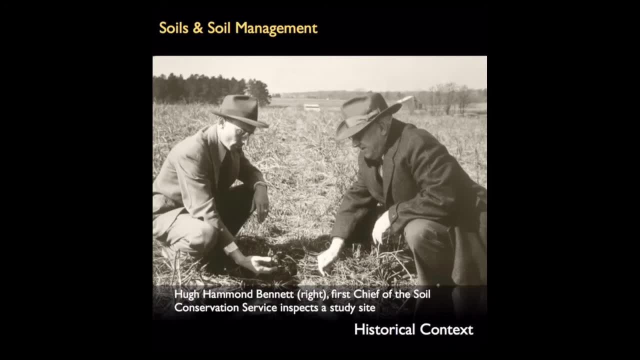 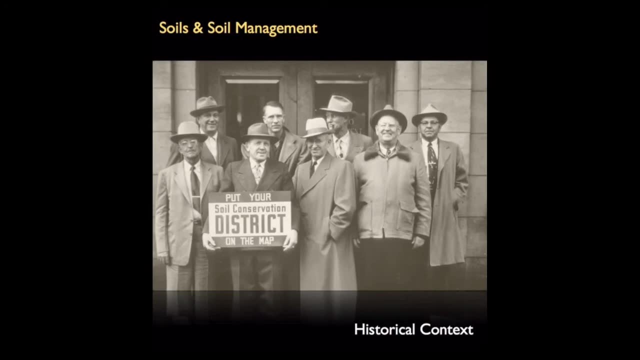 for the development of the soil conservation program, which was a responsible for coordinating research to develop tillage and grazing practices that would reduce soil erosion. These practices were then demonstrated to farmers and ranchers. The agency was organized into approximately 3,000 soil. 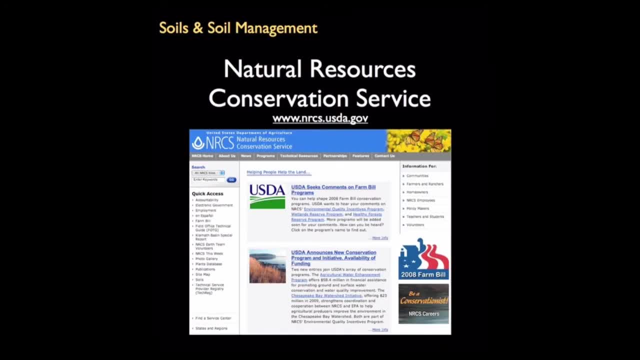 conservation districts and is now called the Natural Resources Conservation Service. The NRCS provides leadership in a partnership effort to help America's private landowners and managers conserve their soil, water and other natural resources. It provides technical assistance in identifying problems associated with soil. 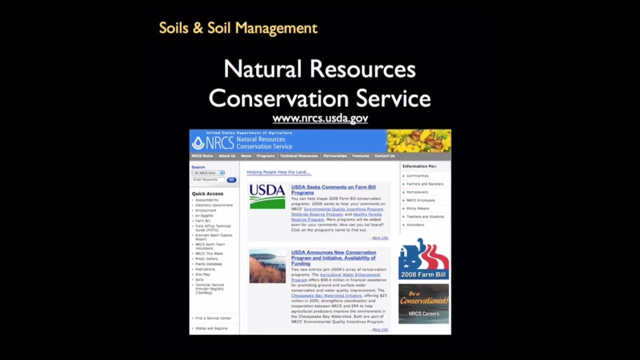 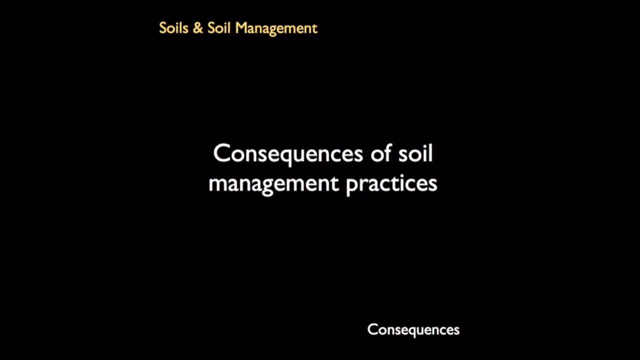 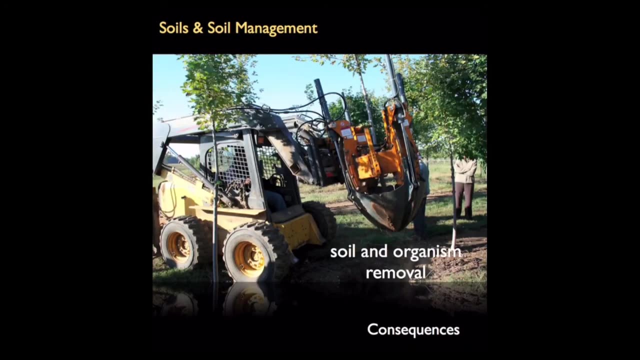 management and develops educational resources that highlight best management practices. Many agricultural activities associated with the growth of plants have profound effects on soil. Crop production interferes with the process of soil formation, first by removing the plants and other organisms that were involved in the process up to that time. Any litter layer of soil that is not 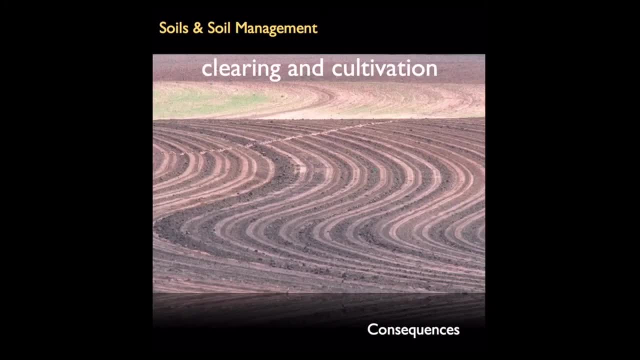 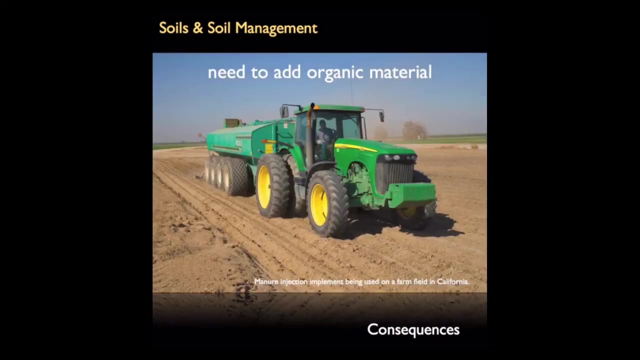 at the soil surface is removed by clearing and cultivation which, if done improperly, can lead to alteration of soil structure by compaction and also leaching, erosion and mineral oxidation. Although crops can add organic matter to the soil, cultivation may increase the rate of microbial decomposition and the net loss of soil is not made up by deliberate 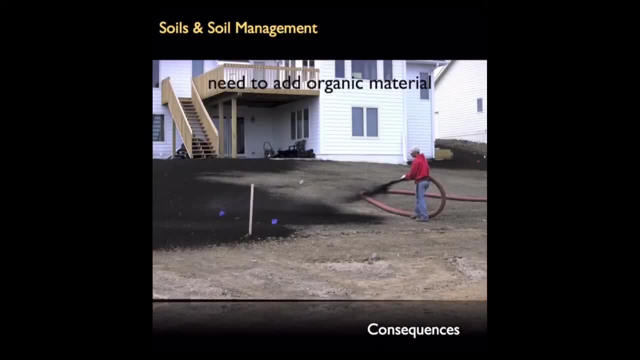 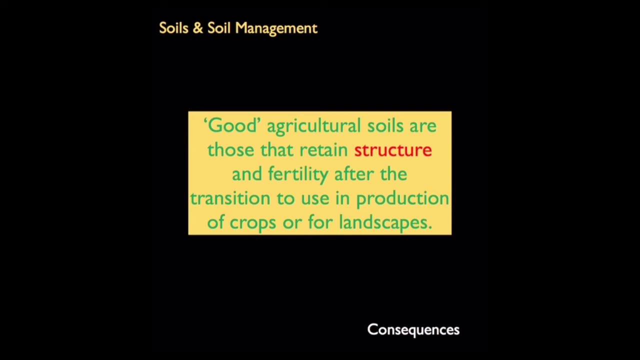 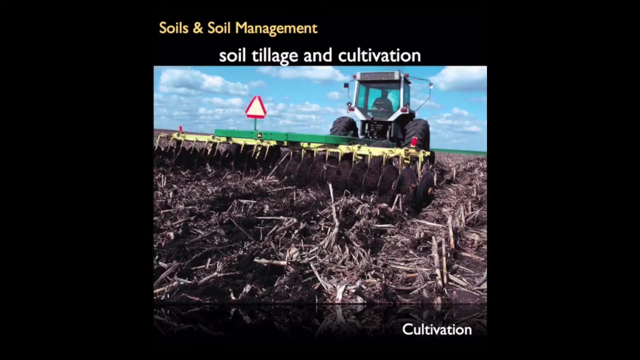 addition of organics. This ends up being usually less than would have come from the native organisms. Good agricultural soils are those that retain structure and fertility after the transition to use in production of crops or for landscapes. One of the principal soil management activities is land preparation for planting. This entails the turning or stirring of soil. 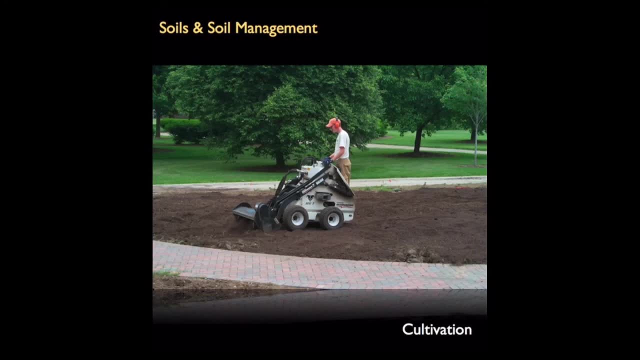 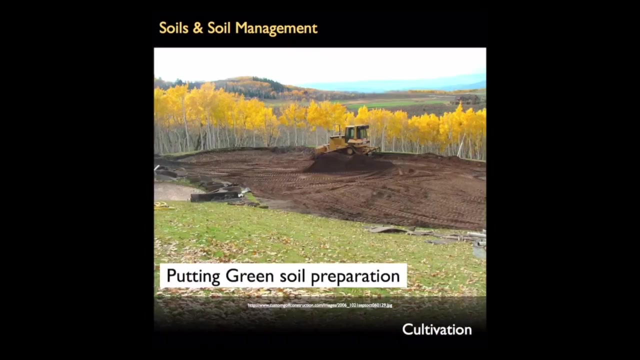 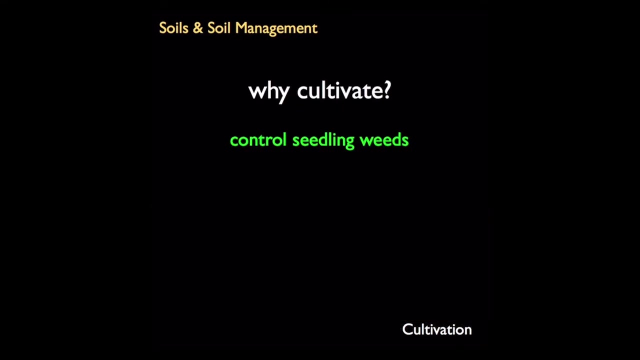 Cultivation of this soil as part of production, installation or management practices is generally considered to be a beneficial soil practice. Cultivation is essential for the establishment and success of constructed landscapes, be they gardens or golf courses and other amenity fields. Soils are cultivated to accomplish four important tasks: to control, seedling, weeds. to incorporate. 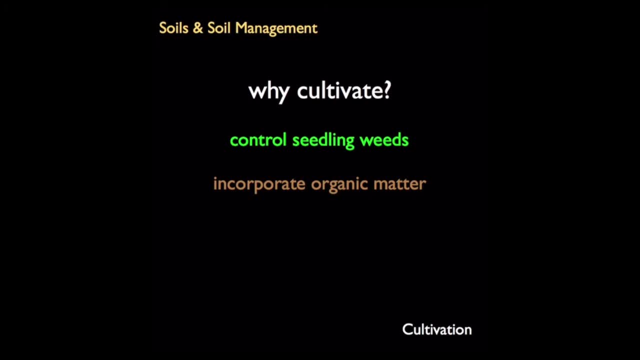 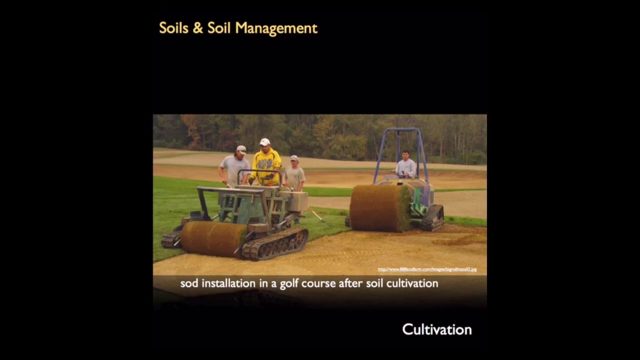 crop or landscape residues to modify soil structure and to prepare ground for seeding or planting. Thus, weed competition can be reduced and soil structure can be improved by breaking up large aggregates and with added organic matter Under optimal conditions: water retention, drainage, aeration, seed germination and root.